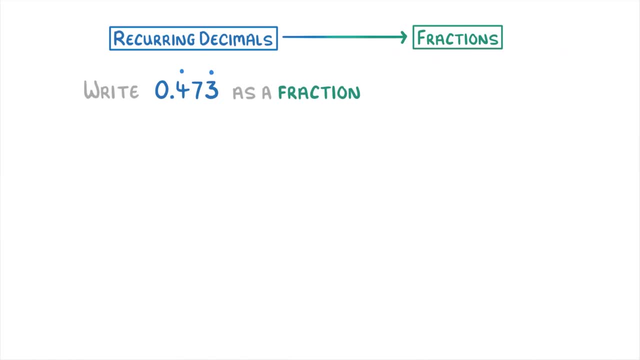 and convert it into a fraction. Before we start, I want to point out that converting recurring decimals into fractions is actually quite complicated and takes a fair few steps, So we're going to work through it slowly, one step at a time. The first thing you want to do is name your decimal with a letter. For example, we might 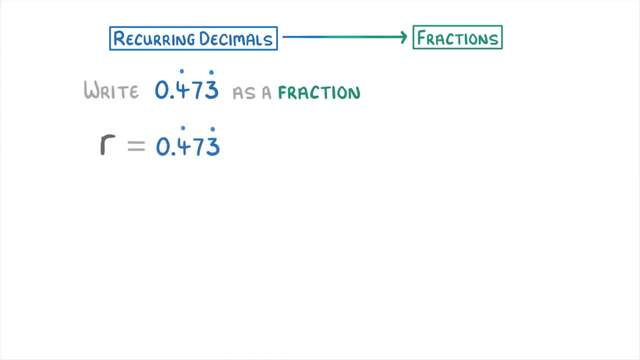 call it R and so write: R equals 0.473 recurring. Next you need to multiply both sides of the equation by 10, until you end up with one entire set of the recurring digits. So we want to end up with a whole set of 473 on the left of the decimal point. 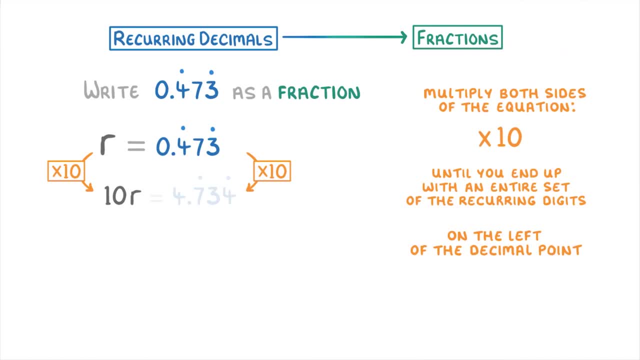 So if we multiply it by 10 once, we'll get: 10R equals 4.734 recurring. times 10 again gives us 100R equals 47.347 recurring, and times 10 once more gives us 1000R equals 400R. 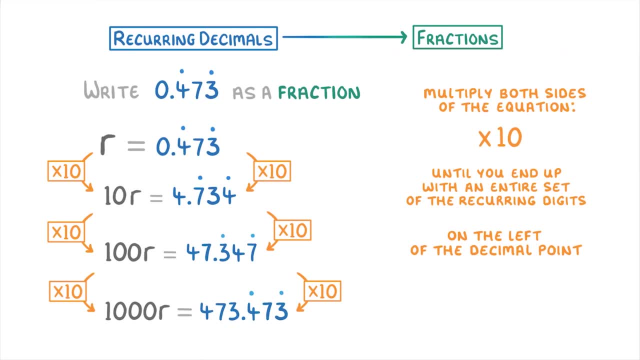 So we're going to multiply both sides of the equation by 10, and so write R equals 0.473 recurring, and so write R equals 0.473 recurring. and so write R equals 0.473 recurring. and so we end up with a full set of the recurring digits. 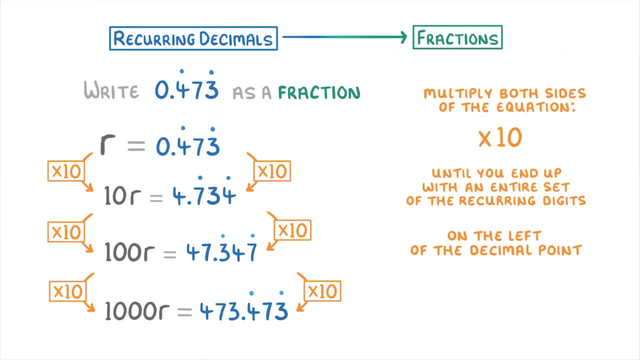 So we now have a full copy of the recurring digits to the left of the decimal point, and so we can stop multiplying by 10.. And to give ourselves some more space, let's just rewrite this up here. Next, if we now subtract a single R- which, remember, has a value of 0.473, recurring from: 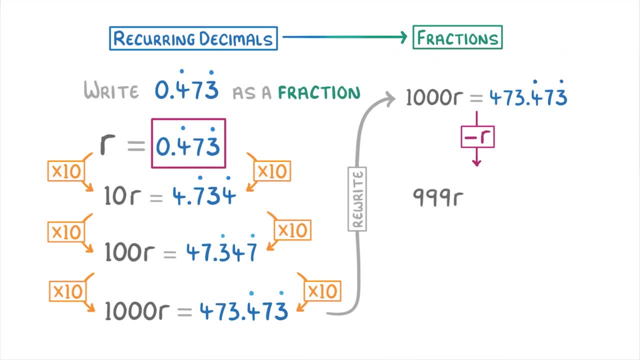 that 1000R, we'll be left with 900R. So we're going to be left with 900R. So if we now subtract a single R, which, remember, has a value of 0.473, recurring from that, But importantly, we'll have completely removed the recurring decimal places from. 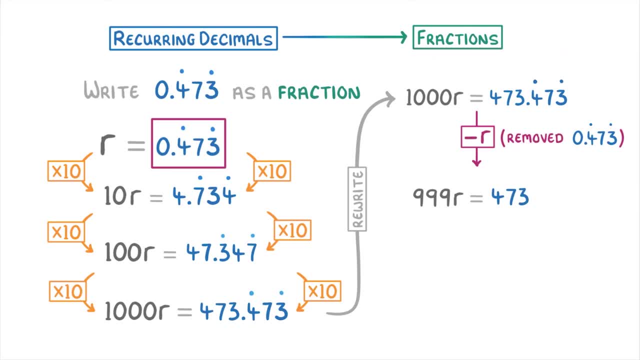 our equation, and so we'll only have 473 left. And because we only have whole numbers in this equation, now to get a single r by itself, all we have to do is divide both sides by 999, which gives us r equals 473 over 999.. 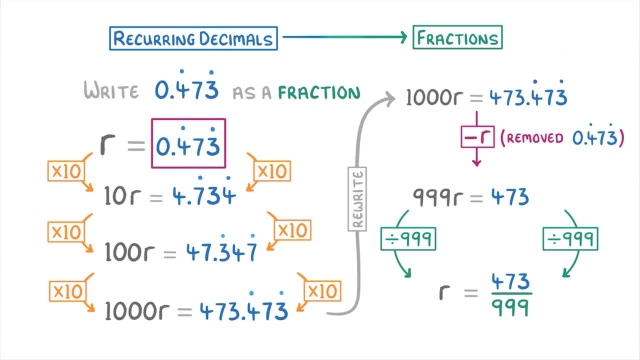 And remember, because r is just a letter, that represents 0.473 recurring- we're really writing: 0.473 recurring is equal to 473 over 999.. And so that's our answer. We've converted that recurring decimal into a fraction. 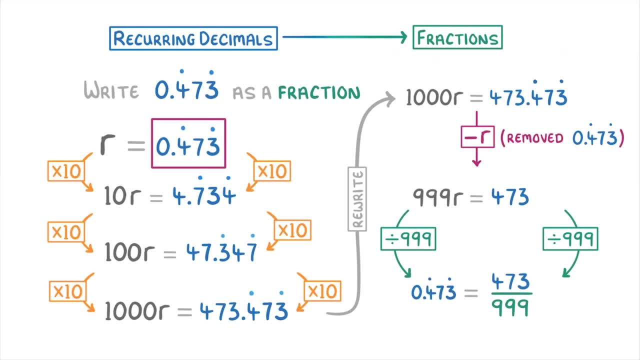 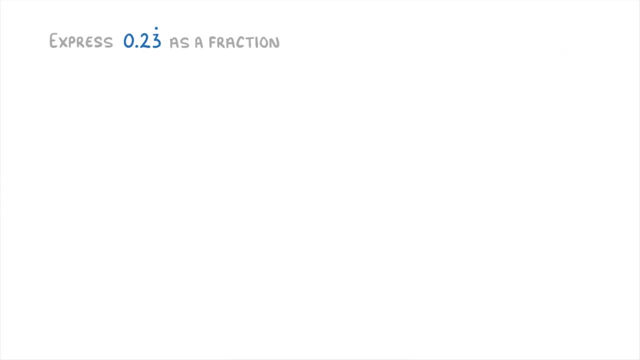 We just had to go through all of these weird steps to get here. Now sometimes you might have a recurring decimal where the recurring part doesn't come right after the decimal point, like in 0.23 recurring where only the 3 recurs. 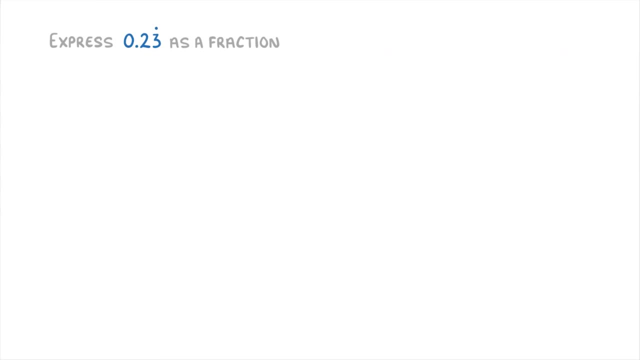 In these cases we have to use a slightly different technique. We still name our decimal r, but this time we write two extra sums. In the first we multiply it by 10 until one whole set of the recurring decimals are to the left of the decimal. 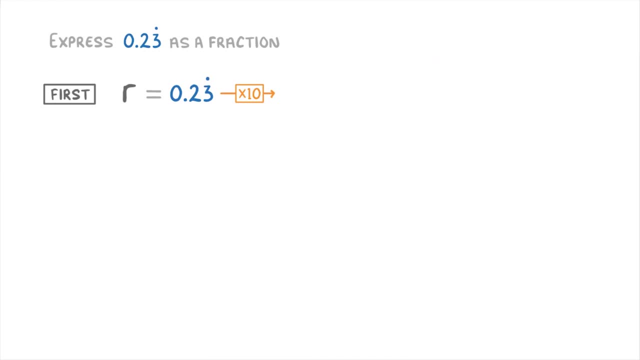 Just like we did last time. So here we'd end up having to multiply by 10 once to get 10r equals 2.3 recurring, and then again to get 100r equals 23.3 recurring. For the second sum, though, we only multiply it by 10 until the non-recurring decimals. 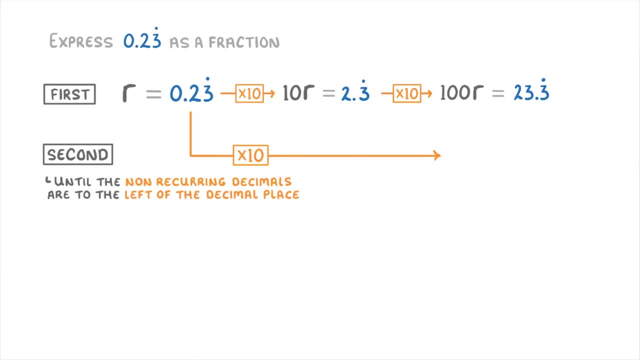 are to the left of the decimal point. So in this case it's just the 2 that we want on the left, Meaning that we only need to multiply it by 10 once to get. 10r equals 2.3 recurring. 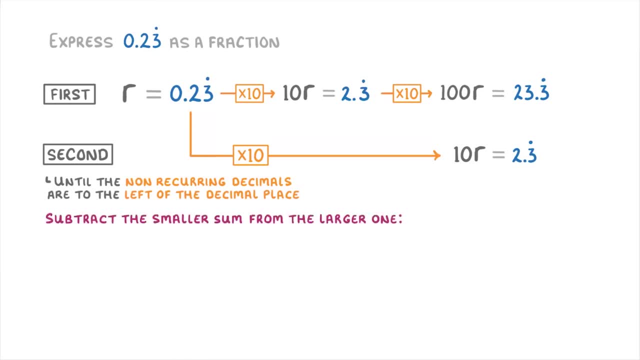 Next we subtract the smaller sum from the larger one. So 100r equals 23.3 recurring. minus 10r equals 2.3 recurring. And for things like this, where you're subtracting one entire equation from another, you just 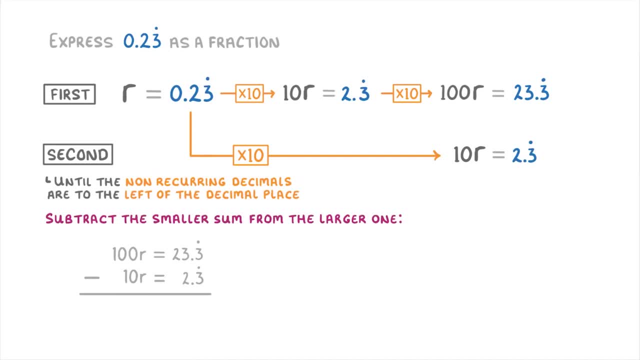 do the left side first and then the right side. So 100r minus 10r is 90r and 23.3 recurring minus 2.3 recurring is 21.. Meaning that we end up with 90r equals 21..